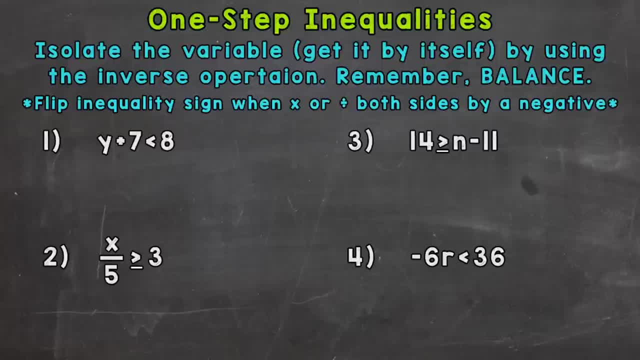 An equation is going to have exactly one solution. So you'll see what I mean as we go through the four examples there on the screen. Now we do need to remember we flip the inequality symbol when we multiply or divide both sides by a negative number. 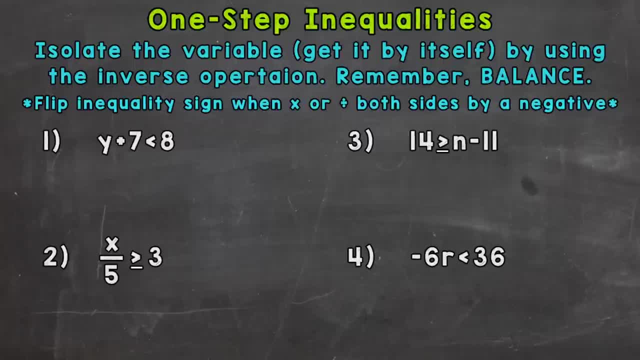 And we have one example of that in this video. So let's jump into number one, where we have y plus seven is less than eight, So we need to isolate our variable of y. We're adding seven to y, So the opposite would be to subtract seven. 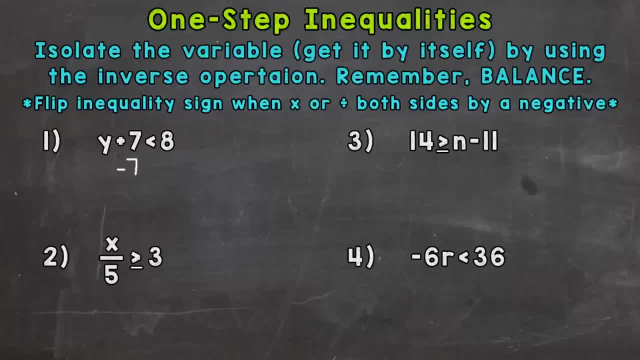 So let's subtract seven from that side And that's going to cancel those sevens out and isolate our y. Now, whatever we do to one side, we have to do to the other. So if we subtracted seven on the left, we need to subtract seven on the right. 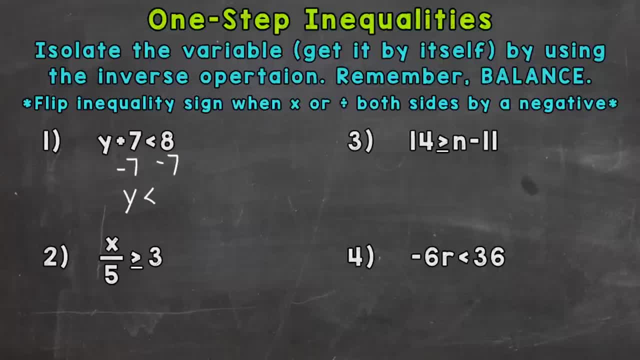 And we add seven to the right And we end up with y is less than eight minus seven is one. So here is our answer: Y is less than one. So any number less than one would be a solution to that inequality. And let's try and test one out here. 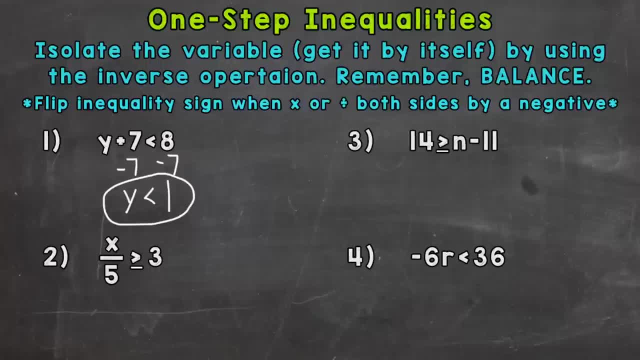 So zero is less than one. Let's see if that works. Let's plug in zero for y, So we'll have: zero plus seven is less than eight. Well, zero plus seven is seven, And seven is less than one, So zero is less than eight. 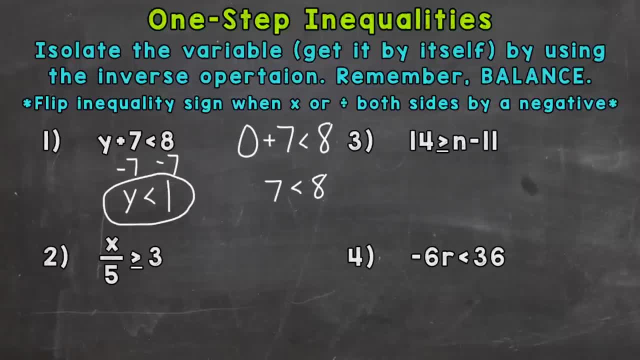 So zero was a solution, along with anything else less than one, An infinite amount of solutions. On to number two, where we have x divided by five is greater than or equal to three, So we're dividing by five. The opposite of dividing by five would be multiplying by five. 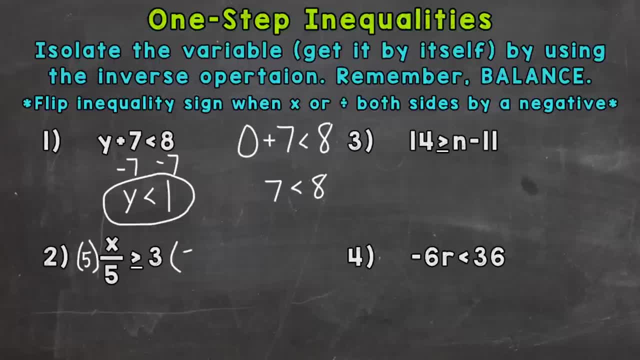 So let's multiply both sides by five. The fives on the left cancel out isolating. So we have x, and we have x is greater than or equal to three times five is 15.. So x has to be greater than or equal to 15 in order to be a solution to that inequality. 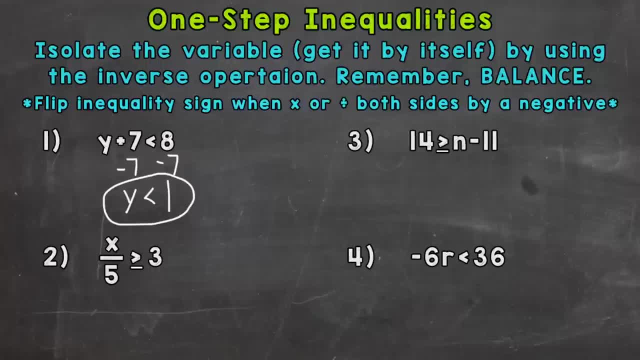 So zero is less than one. Let's see if that works. Let's plug in zero for y, So we'll have: zero plus seven is less than eight. Well, zero plus seven is seven, And seven is less than one, So zero is less than eight. 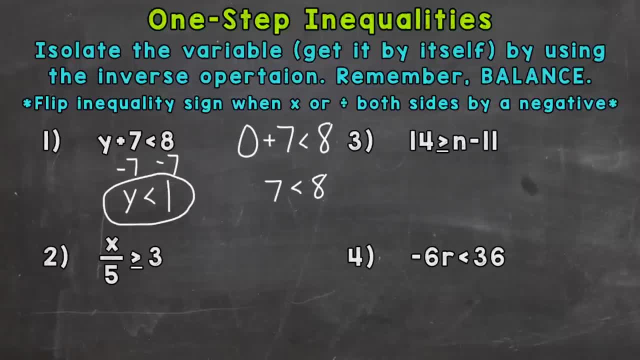 So zero was a solution, along with anything else less than one, An infinite amount of solutions. On to number two, where we have x divided by five is greater than or equal to three, So we're dividing by five. The opposite of dividing by five would be multiplying by five. 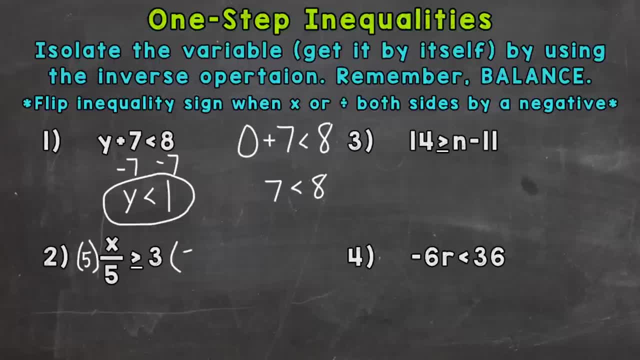 So let's multiply both sides by five. The fives on the left cancel out isolating. So we have x, and we have x is greater than or equal to three times five is 15.. So x has to be greater than or equal to 15 in order to be a solution to that inequality. 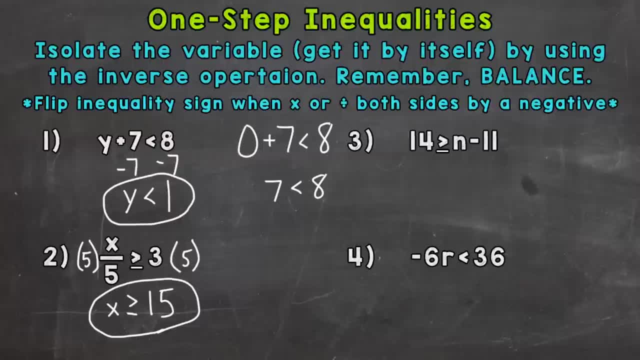 So let's try something out that's greater than 15.. Let's try 20.. 20 divided by five is greater than or equal to three. So 20 divided by five is four. Four is greater than or equal to three. So that's true. 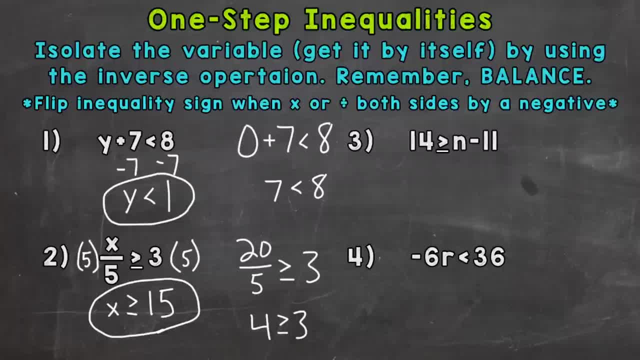 20 would be a solution. Now, 15 is included in the solutions for number two because it's an or equal to inequality. On to number three, where we have, 14 is greater than or equal to n minus 11.. So we need to isolate the n. 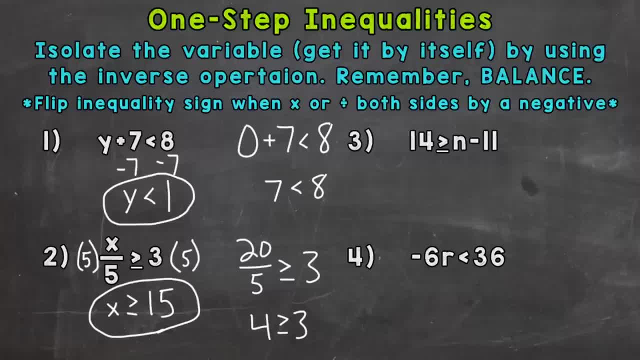 11 is being subtracted from n, So the opposite would be adding 11.. So let's add 11 to both sides In order to isolate the n and keep everything balanced. So n is isolated and 14 plus 11 is 25.. 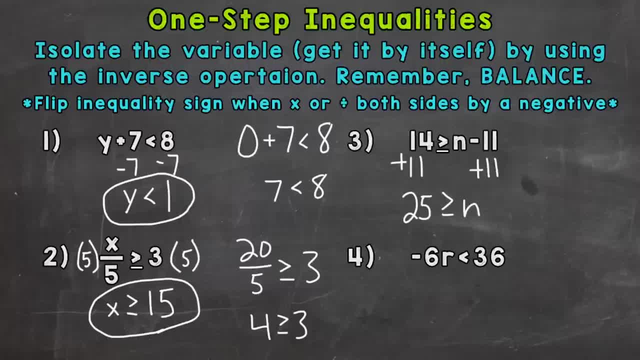 So 25 is greater than or equal to n. So n has to be less than 25 there or equal to 25.. So let's test something out and see if it works. Let's do 20.. 20 is less than 25.. 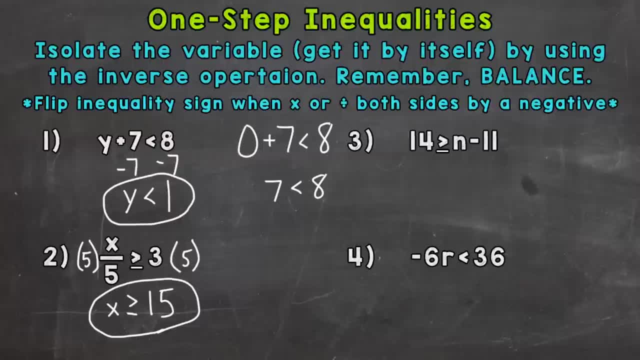 So let's try something out that's greater than 15.. Let's try 20.. 20 divided by five is greater than or equal to three. So 20 divided by five is four. Four is greater than or equal to three. So that's true. 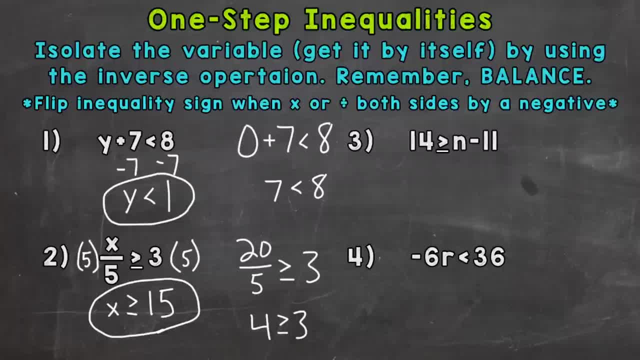 20 would be a solution. Now, 15 is included in the solutions for number two because it's an or equal to inequality. On to number three, where we have, 14 is greater than or equal to n minus 11.. So we need to isolate the n. 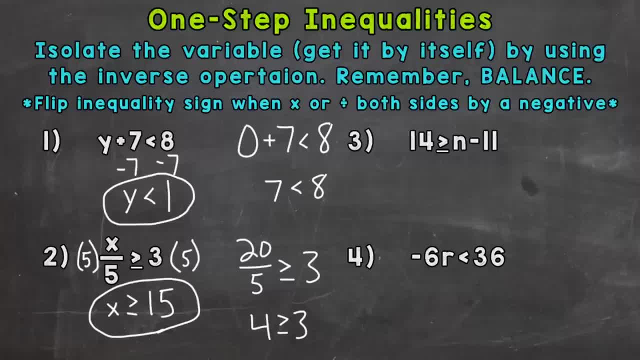 11 is being subtracted from n, So the opposite would be adding 11.. So let's add 11 to both sides In order to isolate the n and keep everything balanced. So n is isolated and 14 plus 11 is 25.. 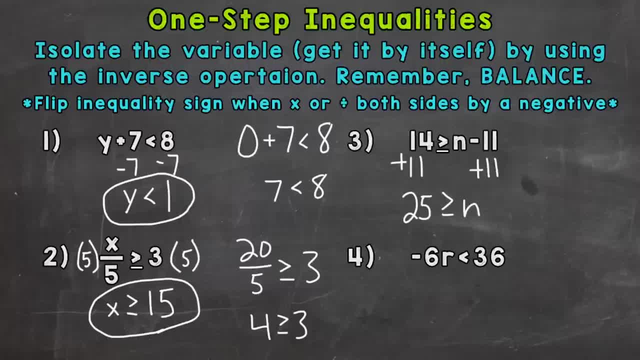 So 25 is greater than or equal to n. So n has to be less than 25 there or equal to 25.. So let's test something out and see if it works. Let's do 20.. 20 is less than 25.. 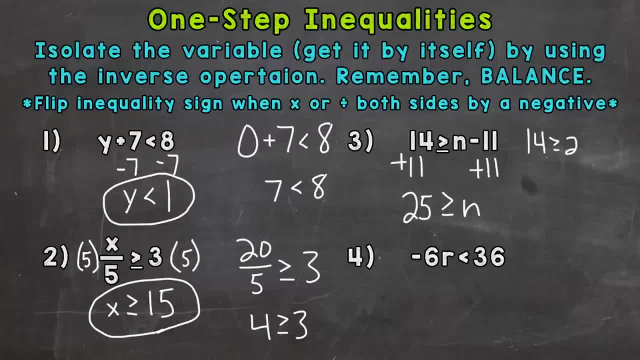 So we will plug 20 in for n. So we have: 14 is greater than or equal to 20 minus 11 is nine, And that is true. So 20 would be a solution, along with anything equal to or less than 25.. 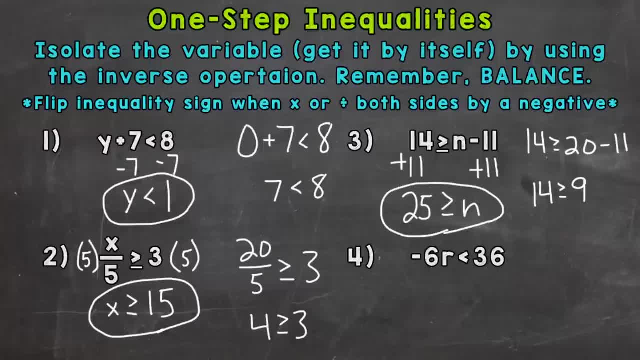 So this is our final answer for number three. And lastly, number four. we have negative six times. r is less than 36.. So we're multiplying r by a negative six. The opposite of multiplying by negative six would be to divide by negative six. 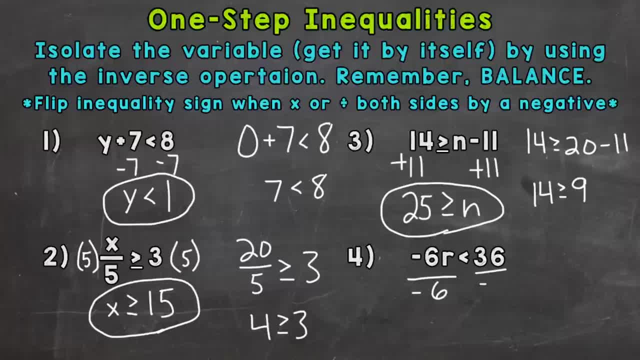 So let's divide both sides by negative six. That cancels the negative sixes out on the left, isolating the r, And we needed to do it to both sides to keep everything balanced. So we're left with r And we need to flip the inequality sign when we multiply or divide both sides by a negative. 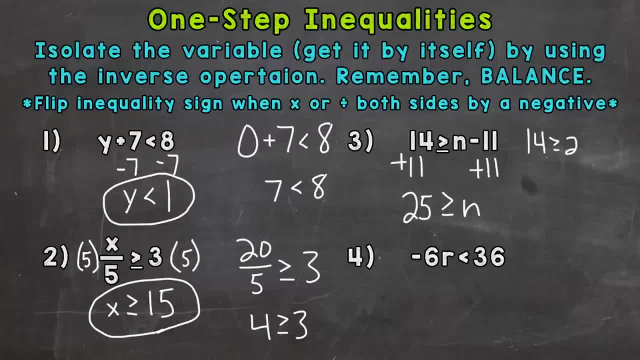 So we will plug 20 in for n. So we have: 14 is greater than or equal to 20 minus 11 is nine, And that is true. So 20 would be a solution, along with anything equal to or less than 25.. 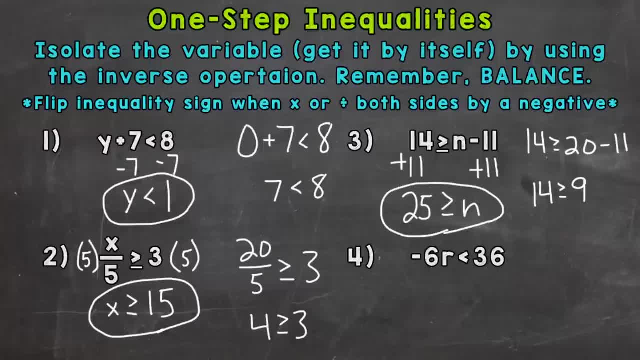 So this is our final answer for number three. And lastly, number four. we have negative six times. r is less than 36.. So we're multiplying r by a negative six. The opposite of multiplying by negative six would be to divide by negative six. 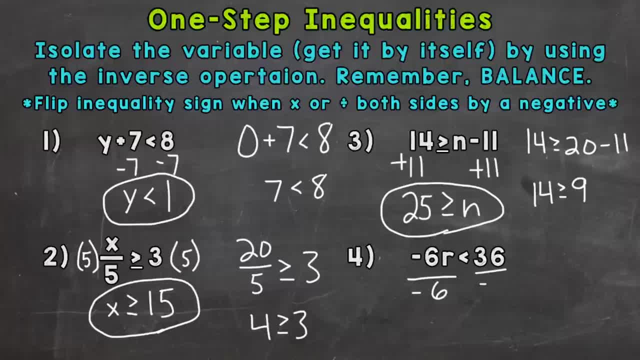 So let's divide both sides by negative six. That cancels the negative sixes out on the left, isolating the r, And we needed to do it to both sides to keep everything balanced. So we're left with r And we need to flip the inequality sign when we multiply or divide both sides by a negative. 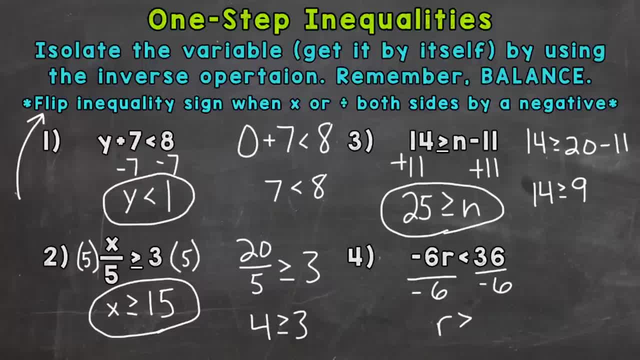 So we need to flip that sign. And 36 divided by negative six is negative six. So r is greater than negative six. So anything greater than negative six is going to make that inequality true. It's going to be a solution. So let's try out negative two. 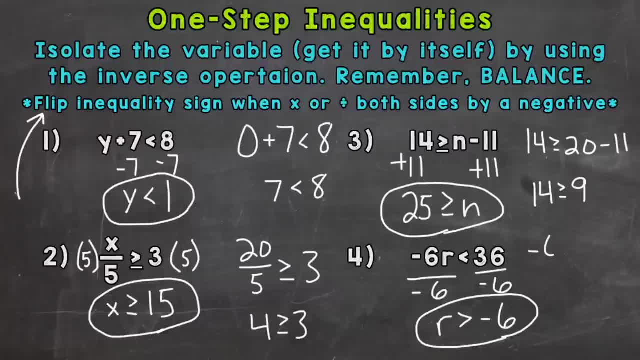 Negative two is greater than negative six. So let's plug that in: Negative six times negative two is less than 36.. Well, negative six times negative two is a positive 12,, which is less than 36.. So negative two would be a solution, along with anything else that is greater than negative six. 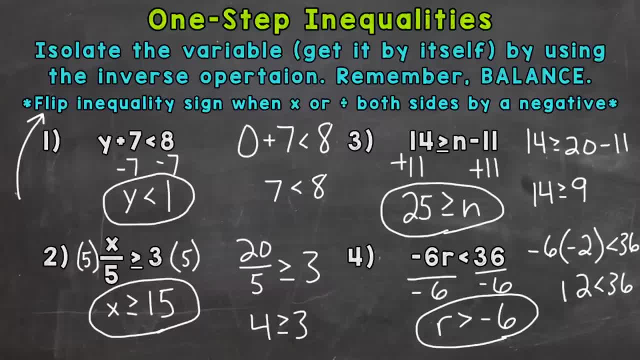 Now, the reason we flip that inequality sign is because flipping the sign will make the inequality true. Without flipping it, we're actually going to get incorrect solutions, the opposite of what we want. And I go into further depth about why we flip that sign and more examples in some different videos. 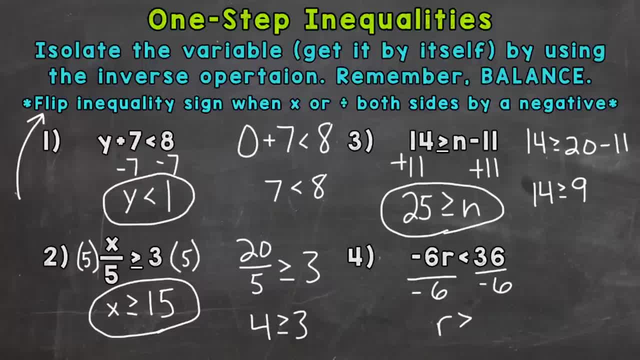 So we need to flip that sign. And 36 divided by negative six is negative six. So r is greater than negative six. So anything greater than negative six is going to make that inequality true. It's going to be a solution. So let's try out negative two. 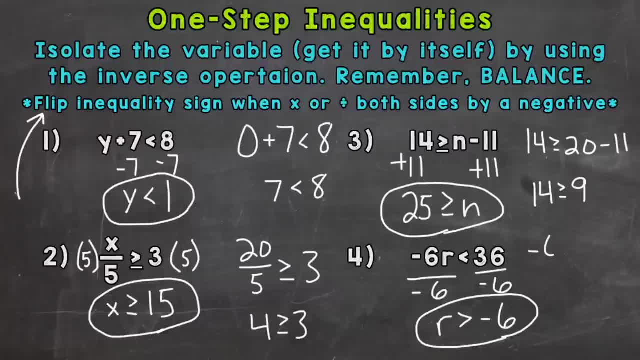 Negative two is greater than negative six. So let's plug that in: Negative six times negative two is less than 36.. Well, negative six times negative two is a positive 12,, which is less than 36.. So negative two would be a solution, along with anything else that is greater than negative six. 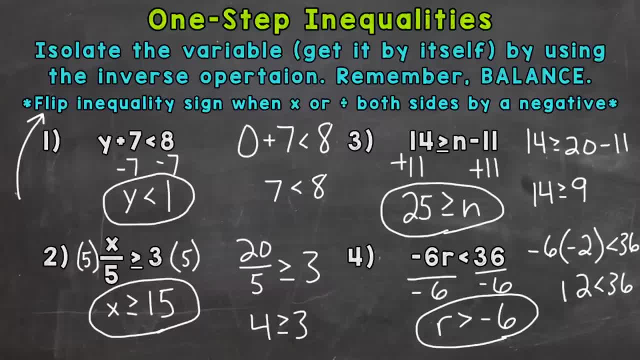 Now, the reason we flip that inequality sign is because flipping the sign will make the inequality true. Without flipping it, we're actually going to get incorrect solutions, the opposite of what we want. And I go into further depth about why we flip that sign and more examples in some different videos. 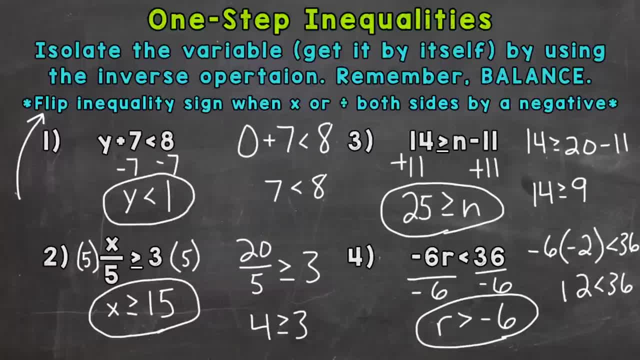 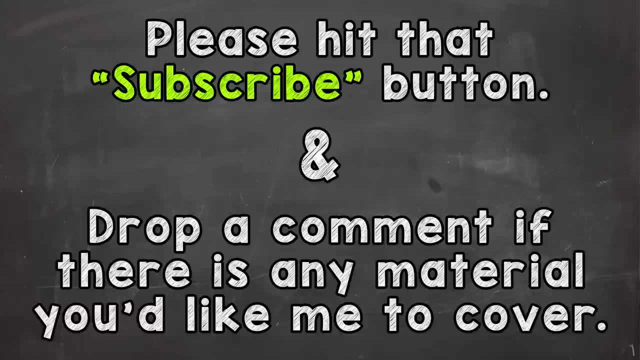 I'll drop those links down in the description. So there you have it. There's how you solve one step inequalities. I hope that helped. Thanks so much for watching. Until next time, Peace. 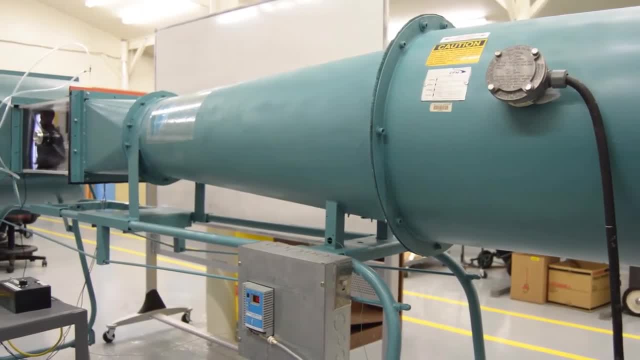 WIN stands for wind tunnel integration of new data acquisition systems. 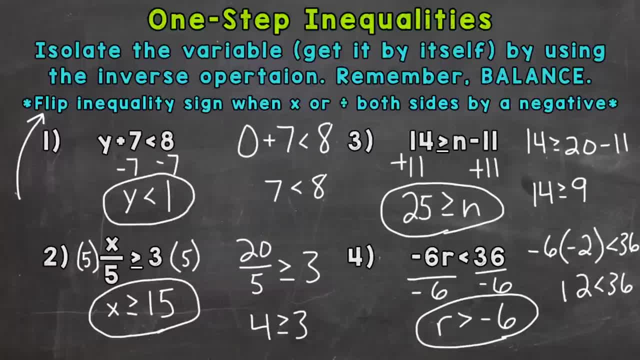 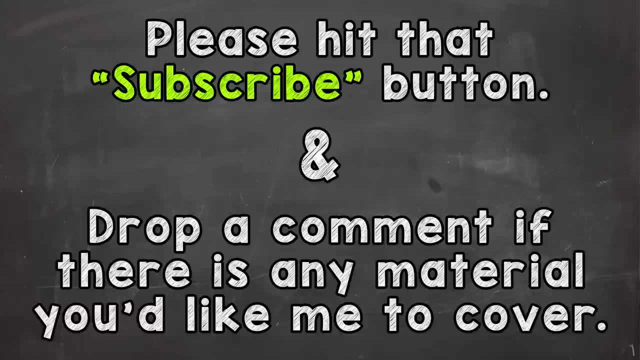 I'll drop those links down in the description. So there you have it. There's how you solve one step inequalities. I hope that helped. Thanks so much for watching. Until next time, peace.